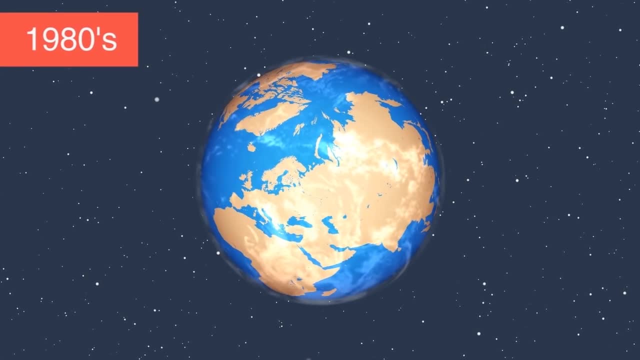 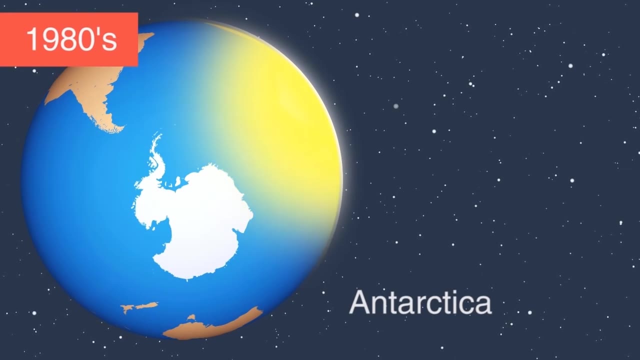 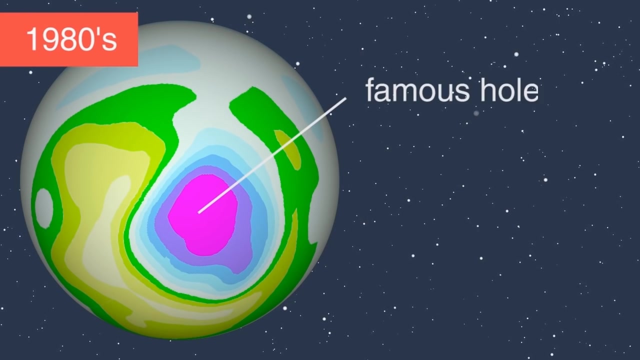 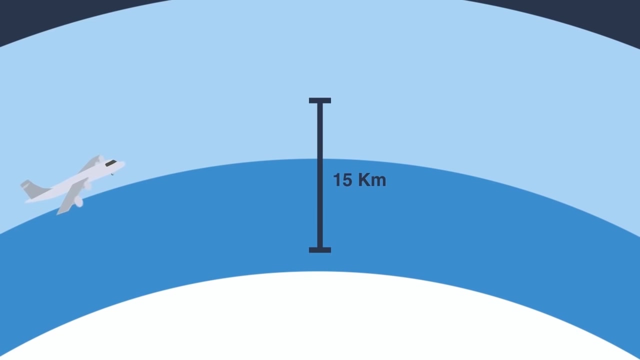 the ground view part A of this video. In the 1980s, scientists found something alarming happening over Antarctica during October, when the sunlight returns to the South Pole after winter. The ozone had almost disappeared over large areas, causing the famous hole. An aircraft which analyzed the composition of the air flew due south, 15 km above the. 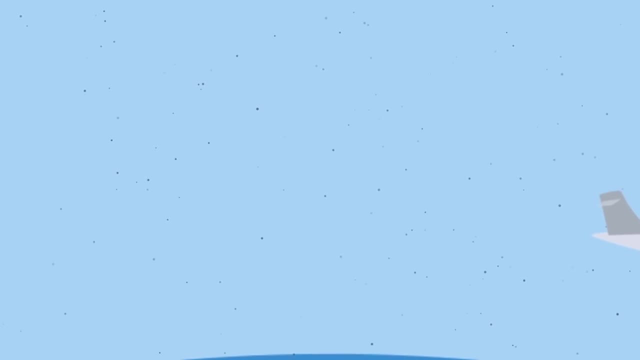 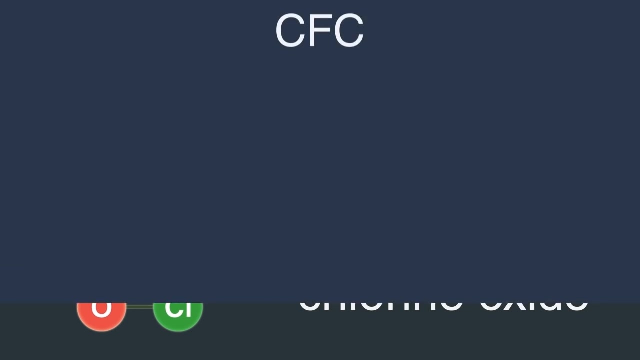 Earth, in the stratosphere, where the ozone is made, They found that the ozone there suddenly became replaced by chlorine oxide. This led to the realization that the chemicals called CFCs- chlorofluorocarbons- were to blame. These 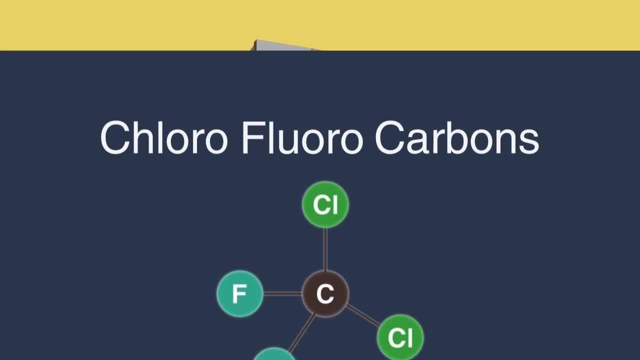 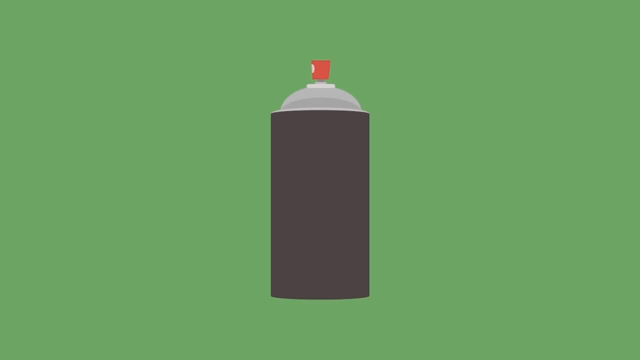 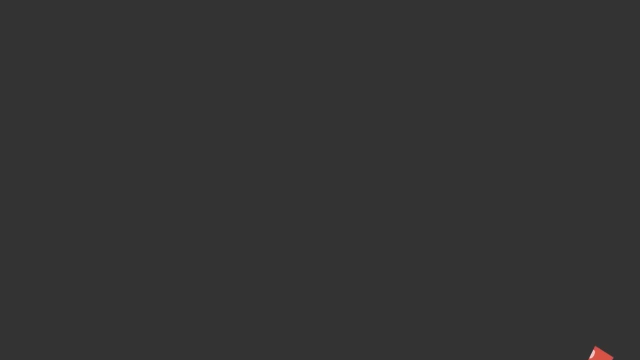 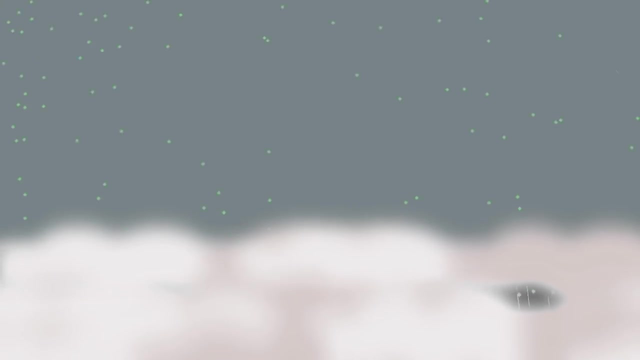 are inert, stable molecules and were once the wonder chemical used as the fluid in fridges and air conditioners to expand polystyrene and in aerosol cans to propel hairspray and paint and so on. They were completely harmless. CFCs are so inert that they do not get washed out in the rain or broken down in the troposphere. 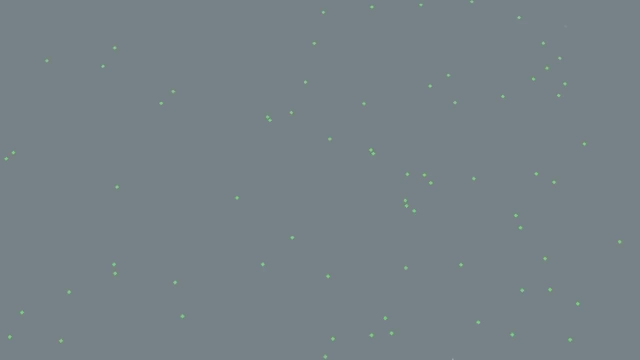 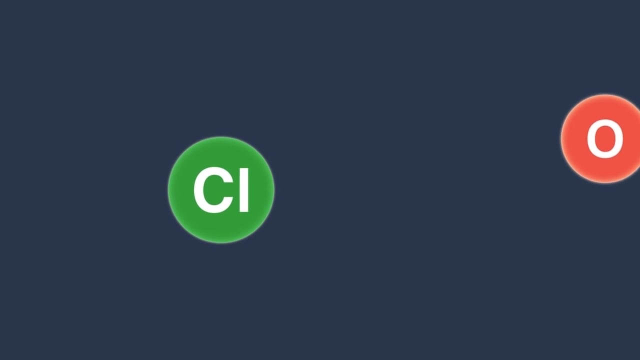 so they diffuse up into the stratosphere. Use your knowledge about how ozone is formed to think about what might happen to CFCs in the stratosphere. Pause and think. Here they are bombarded with ultraviolet light, which breaks chlorine atoms off the molecule. 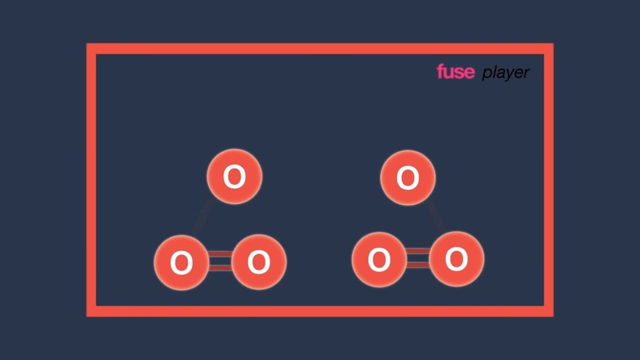 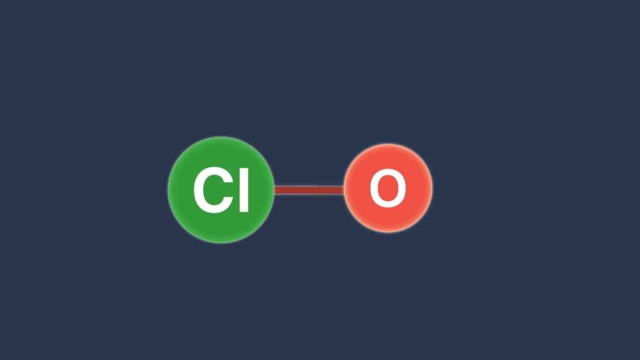 These then bond with the free oxygen atoms, preventing them from reforming ozone in the ozone-oxygen cycle. we saw in the first part of this video. When the chlorine oxide meets yet another oxygen atom, molecular oxygen reforms, leaving the chlorine atom to continue to remove more atomic oxygen. These chlorine atoms are eventually. 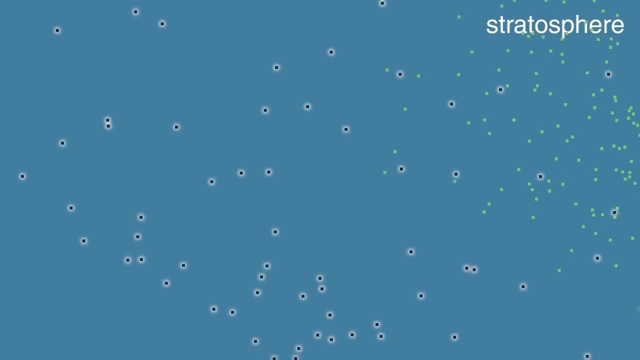 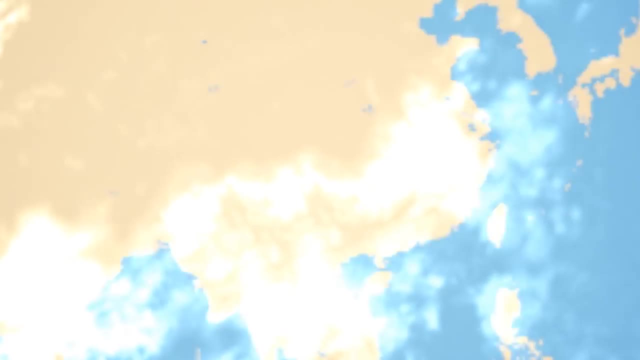 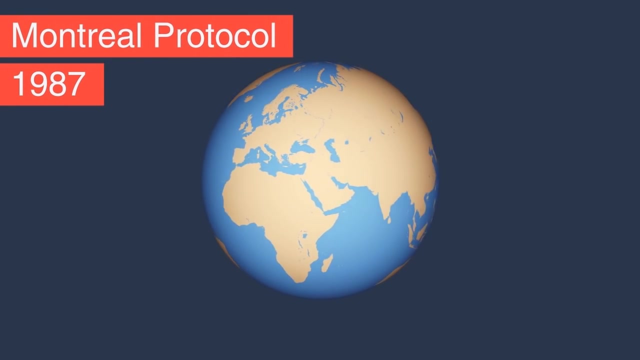 removed from the stratosphere, naturally, but not before they have captured thousands of ozone-forming oxygen atoms. Thus the ozone-oxygen cycle was destroyed and the ozone layer was thinning all over the world. Thus, in 1987, the Montreal Protocol was signed by all nations of the world, banning the production. 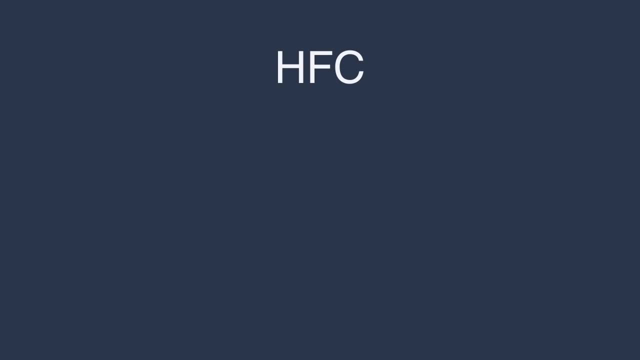 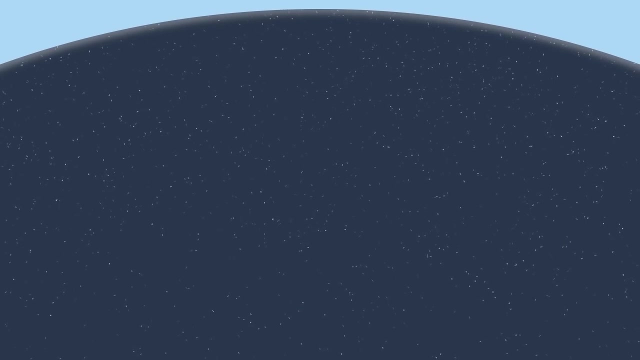 and, eventually, use of CFCs. They have been replaced by HFCs, hydrofluorocarbons, a similar molecule which contains hydrogen in place of chlorine, making them a little more reactive and so able to be broken up in the troposphere before they reach the ozone layer. 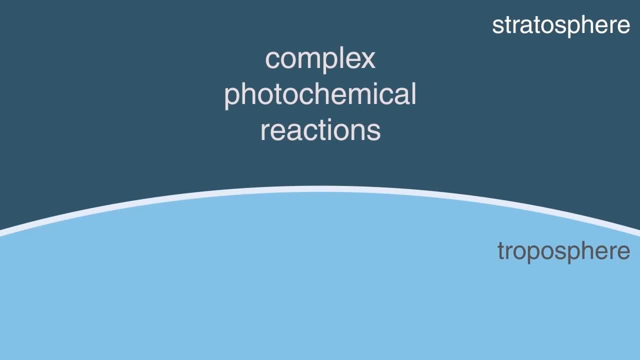 Because the chlorine is slowly and naturally removed from the stratosphere by complex photochemical reactions and because the ozone layer is naturally reforming all the time by the action of UV on oxygen, we expect the ozone to return to its original level in 50 or 100 years time. The hole in the ozone layer allows harmful UV radiation to reach ground level, which can cause skin cancer. However, a common misconception is that it lets heat in and causes global warming, and this is not true. Ozone is also generated in the troposphere by a complex series of photochemical reactions. 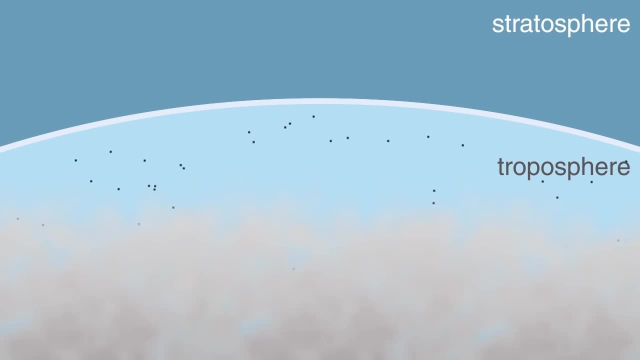 on the products from vehicle exhausts Here in the troposphere. ozone acts as a greenhouse gas and helps in the formation of photochemical smogs that pollute certain cities worldwide from time to time, For example, Los Angeles in the USA. and Beijing in China. 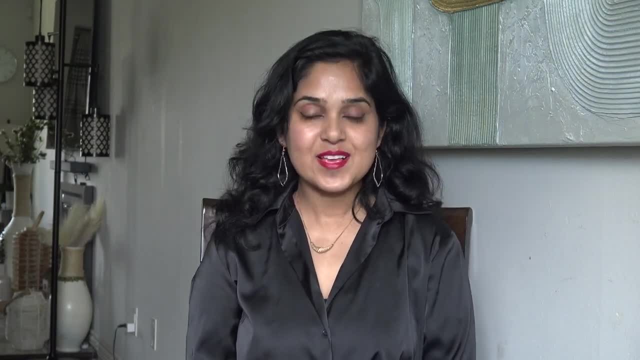 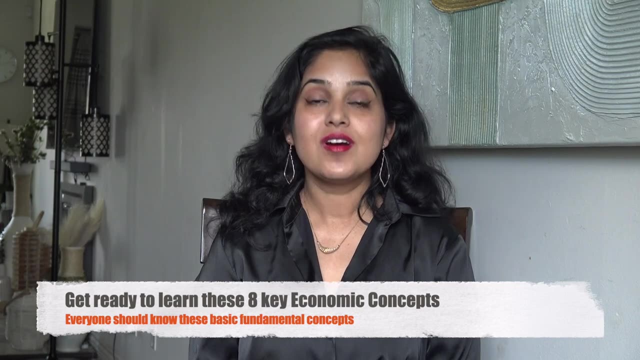 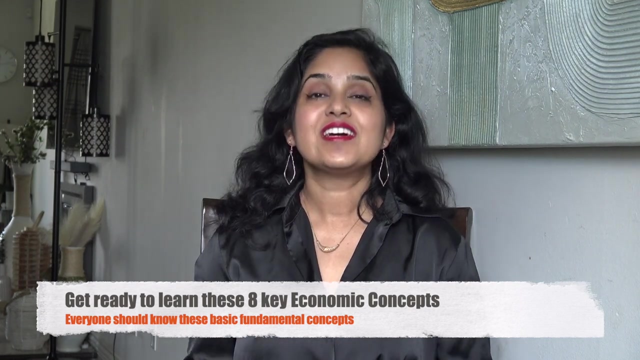 Money makes the world go round, but do you know the economic concepts that make it all possible? In this video, we'll cover the key economic concepts that everyone should know, no matter what their educational background is. From supply and demand to competitive advantage, get ready to expand your economic knowledge and impress your friends with your new insights. 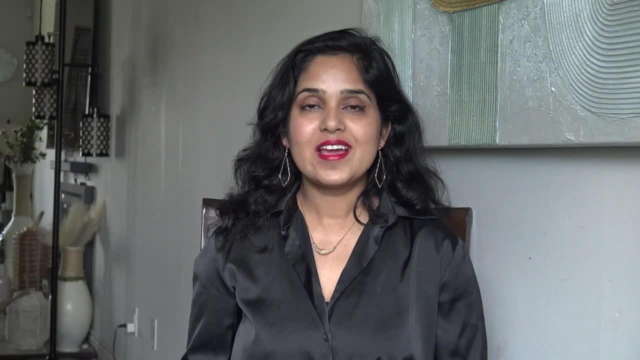 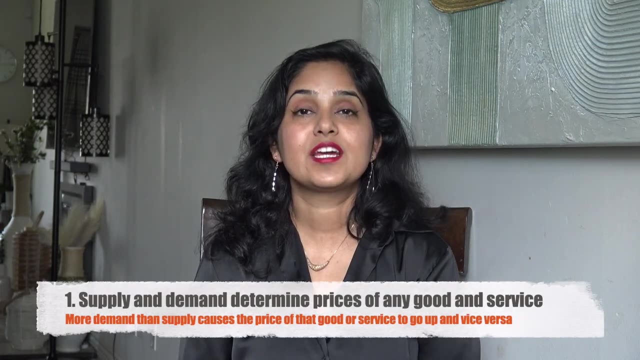 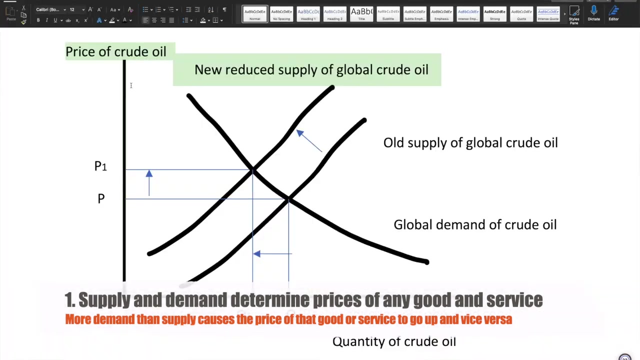 I'll explain these key economic concepts on a very high level so everyone can follow, whatever your educational background might be. The most fundamental concept in economics is of supply and demand. When many people want product and there isn't enough of it, the prices go up. when there is a lot of product and not many people want it, the prices go down. 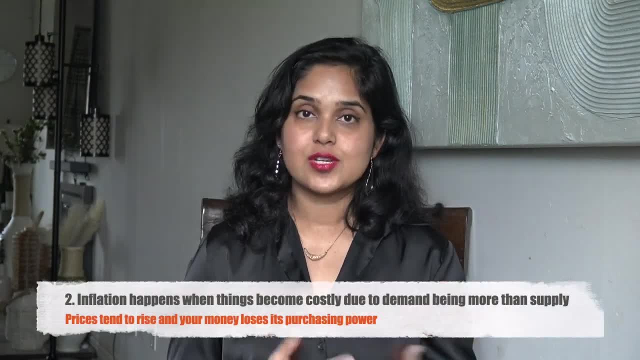 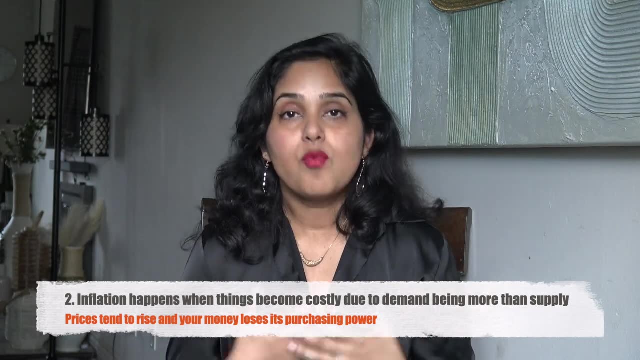 Second closely related topic to supply and demand is inflation. when things cost, the tool to supply and demand is inflation. When things cost less, the products are less more money. over time it's called inflation. This means that the money you have today won't buy as 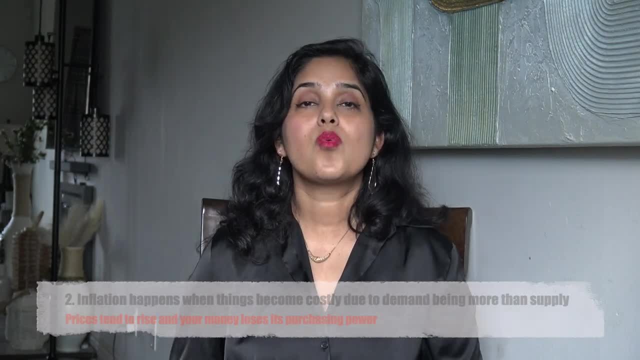 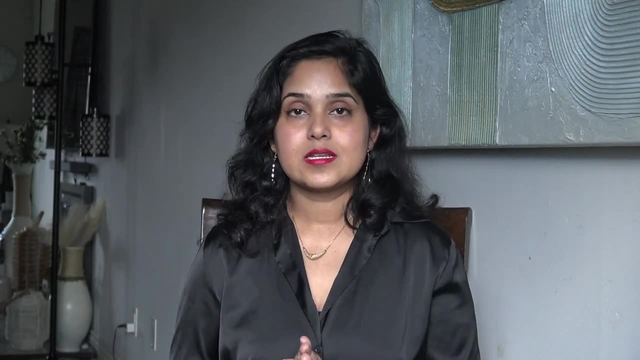 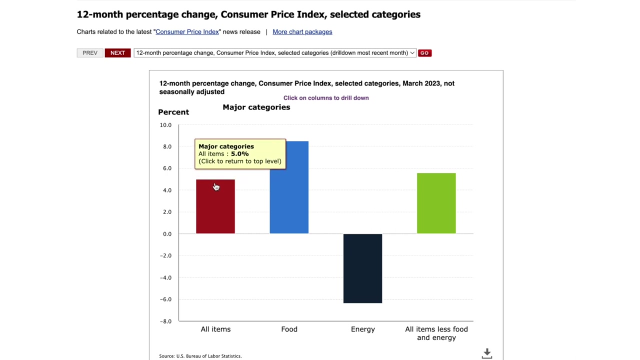 much as it could have in the past. This usually happens when there is more demand than supply of those goods and services, So we usually get inflation numbers in percentages like current US inflation is 5%, which means that the typical goods that you buy and the services that you use 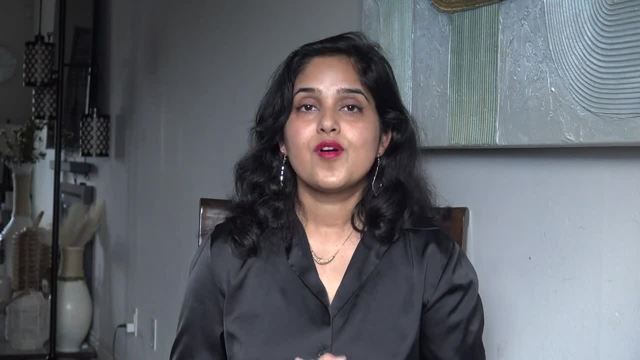 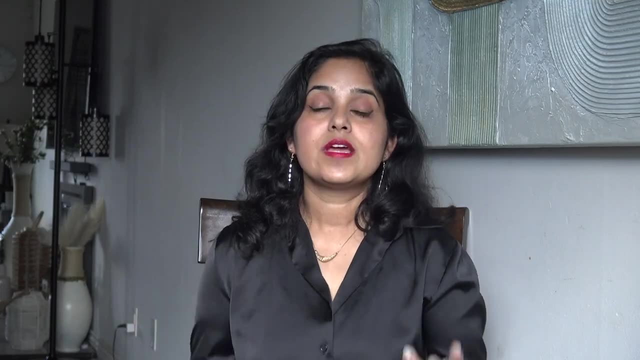 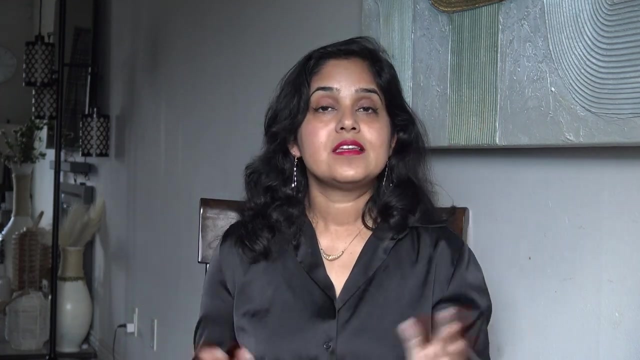 everyone. So understanding inflation is crucial for making informed decisions about investments, saving and your spending. If you want to know more about inflation, I have made several videos on inflation, so you can check those out here. The next concept is called GDP, or gross domestic product. It is like a report card of the economy.